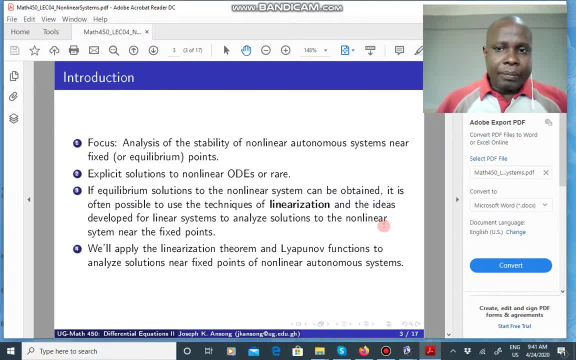 Okay. So, unlike the linear systems that we've looked at, like planar linear systems and so on, where you can actually compute an explicit solution, here it's very rare to have explicit solutions. All right, Okay, And so the mathematical machinery is not as well developed. There are a few things available to us to be able to tackle such problems. 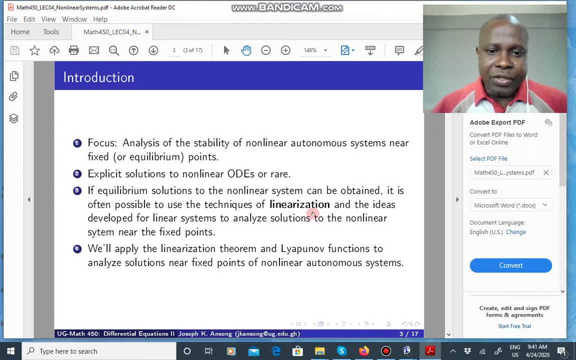 And one of those techniques that we'll be using is called the linearization technique and that is the linearization theorem. And then also, if you are able to get developed layup normal functions, then you can use that to analyze this nonlinear autonomous systems. 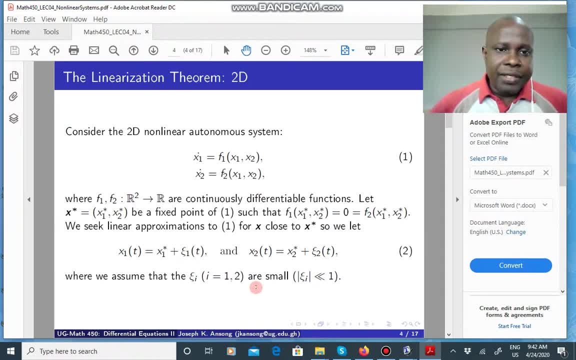 Okay, And so we'll start off with the linearization theorem. This is like a background to it before we actually state the theorem. So we want to consider a two-dimensional nonlinear autonomous systems given by this. So this is a nonlinear, if you like, something like x squared minus y plus xy. 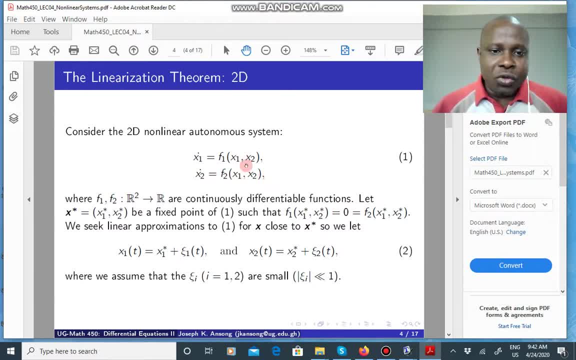 This could be like y squared minus x or something. So f1 and f2 are nonlinear, Okay, Continuously differential. Now if you let x star be given by this right, x1 star, x2 star, let it be a fixed point, such that, well, once it's a fixed point or an equilibrium point, then if you put it into the right-hand side here, this should go to zero and that should go to zero. 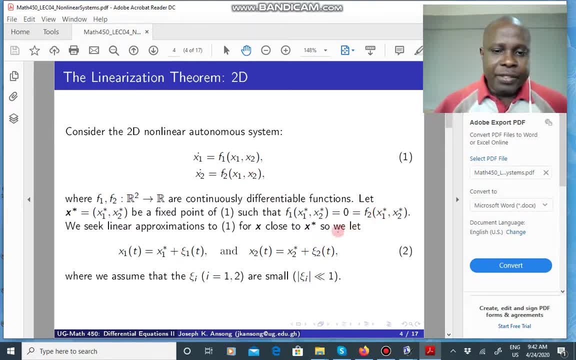 So that's what we have here, All right. So in this case we want to seek solutions around the fixed point. That is the idea of the linearization theorem. You want to look for solutions Not in the whole plane, but you want solutions just around a neighborhood, around the fixed point. 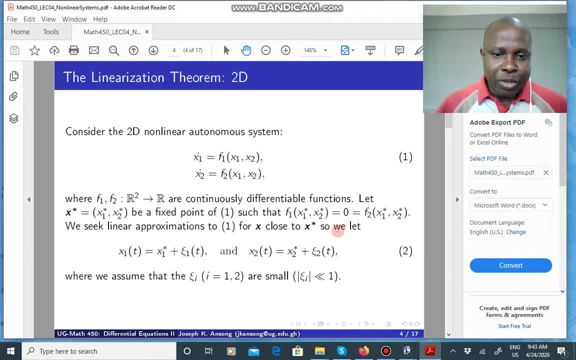 That's all you can do for this technique. So you pick a fixed point which you are calling x star here, and then you expand or linearize about it. Okay, So you let x1 be equal to x1 star, which is your fixed point, plus a small perturbation. 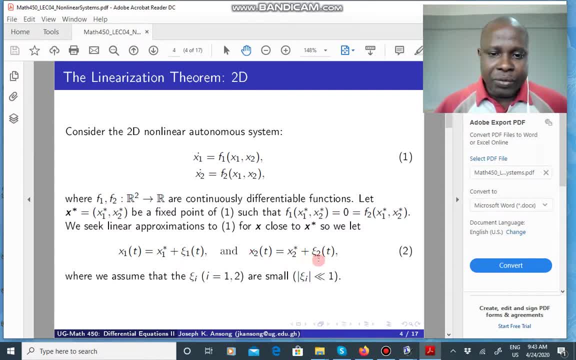 Okay, Xi1.. And then x2 be equal to x2 star plus xi2.. Okay, So this is just a number, right? This is a fixed point. This is a small, you know a small variable. Okay, Xi1 and xi2.. 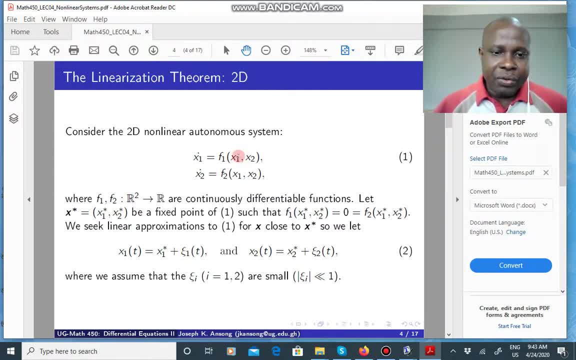 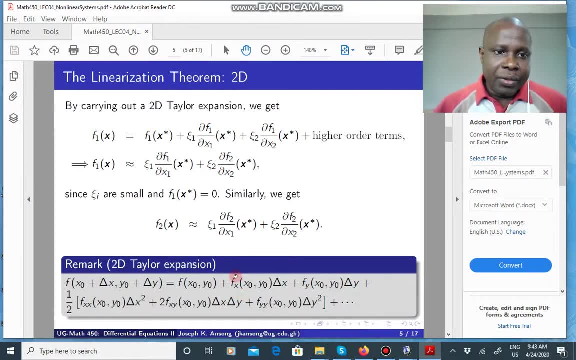 So once you have this, you plug these guys into the right-hand side of this equation and expand them. Okay, So that's what we're going to do. So if you plug so, f1x will be equal to, we are expanding about x star. 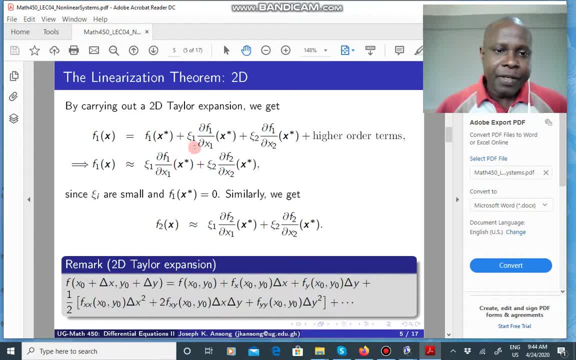 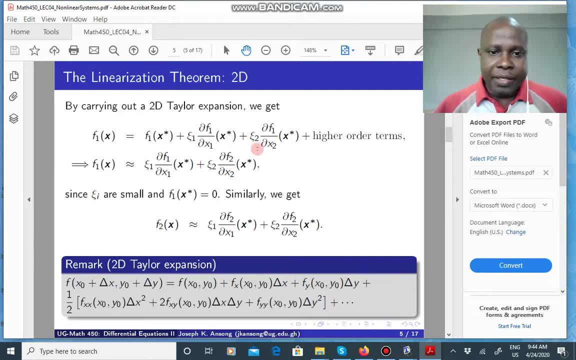 This is x1 star, x2 star Plus. then you get xi2, the derivative of this with respect to x2 at the fixed point, plus higher order times. These higher order times constitute, you know things like they will have terms with xi1. 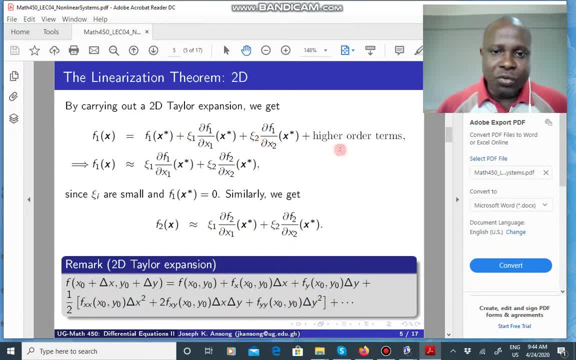 times xi2, or xi1 squared, xi 2 squared. all right, because i1 is small, the square of that or the product of that is also very small, and so you can neglect you can neglect that. and because x star is a fixed point, right f1, x star is of course equal to zero, and so you end up with this. okay, now, if you have forgotten, 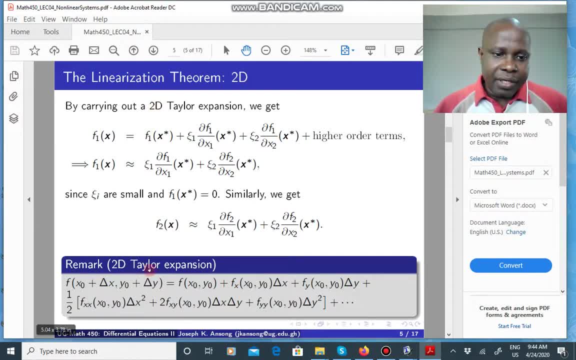 how to do taylor expansions in 2d. this is, this is um. i've written something down here to help you out. so if i'm expanding the function f about x, naught and y naught, um with delta x and delta y. so these are like my xi1 and xi2 and this is like x1 star, x2 star if you expand it. this is what you. 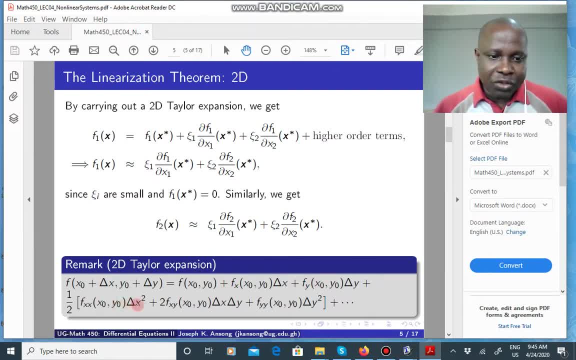 get all right. so these higher order times are these guys, the squares of xi1, the product, the square of xi2. so these are very small. so this is directly that. okay, you can do the same thing for f2. if you do that, you end up with this equation. all right, so we rewrite this: uh, two again. uh now note, note this. 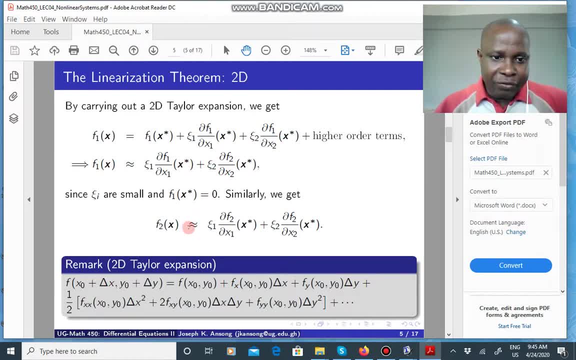 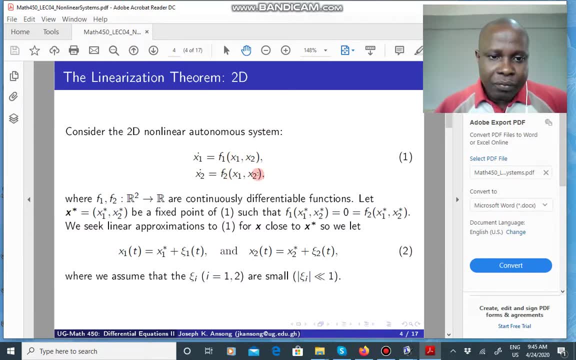 so we have expanded f1 to be this, f2 to be this, if you go back to the original equations so you can plug them back in here, f1 and f2. note that x1 dot does a derivative respect to t. respect to t, this is just a number. so x1 dot is the same as xi1. 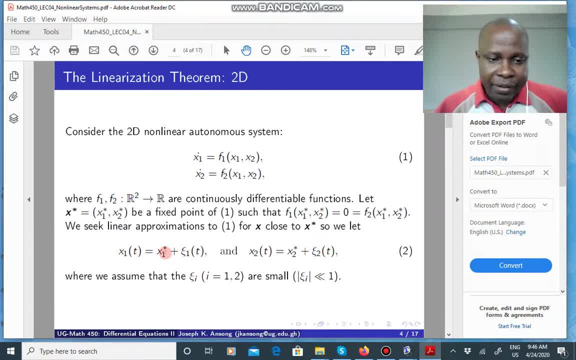 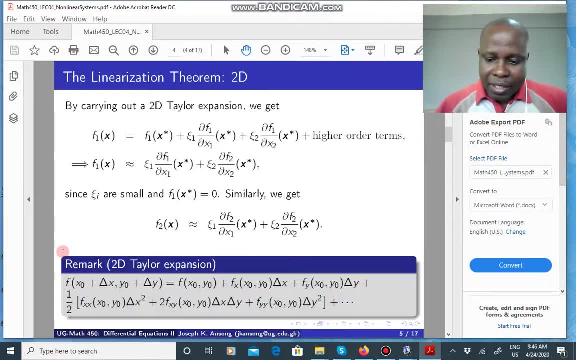 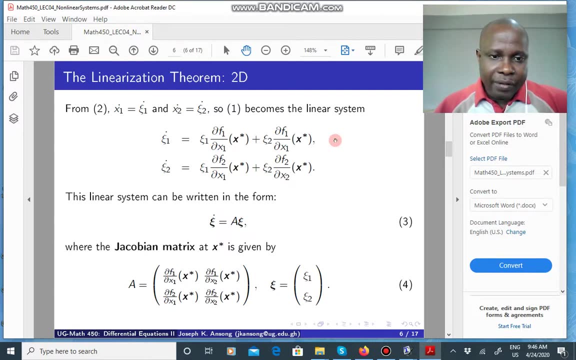 dot, because this goes to zero, because it's just a number, right, it's constant. and then x2 dot is just zeta 2 dot, because this is also constant, so it vanishes. and so we plug f1 and f2 into the original equation and we get this system all right. and so now this is a linear system, because these 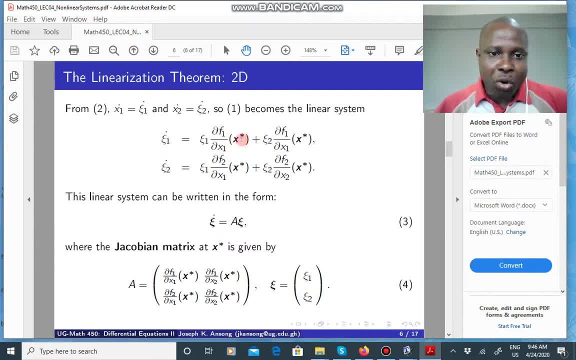 derivatives are evaluated at this point at this number, and so this is just a number, that is a number, this is a number. so these are now. you have converted the non-linear system into a linear system by expanding this into a series. all right, and so these two systems you can rewrite as this, and this is more like the planar system. 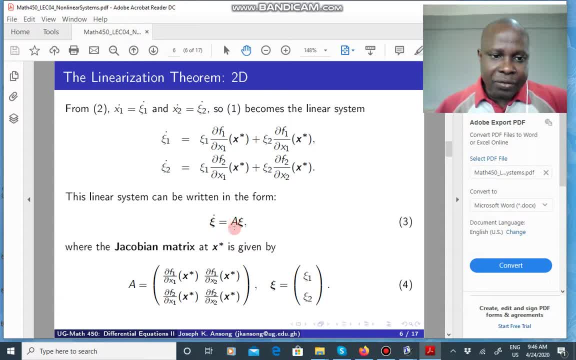 that we have analyzed. okay, and this a is referred to as the jacobian matrix. it's a matrix consistent of the derivatives at the fixed point and, of course, zeta here is zeta 1 and zeta 2.. okay, so by doing a expansion you have changed the non-linear system into a linear system, that we have a machinery that 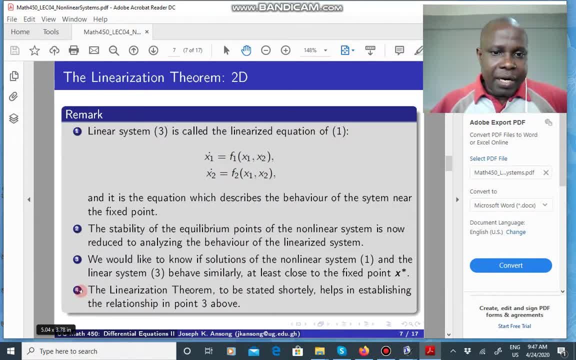 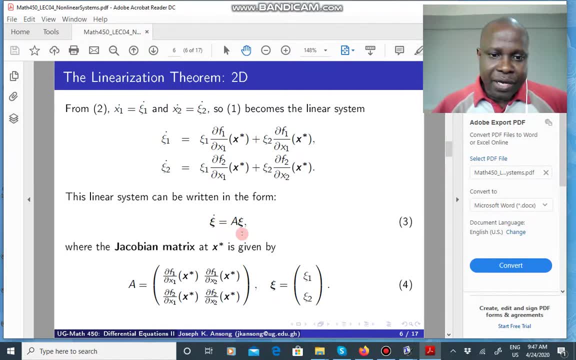 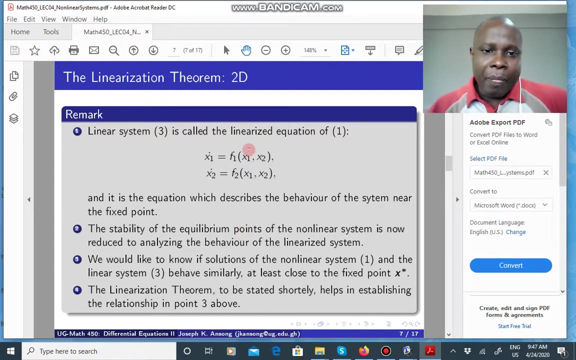 we can analyze, okay, um, so now, uh, this equation here, this linear system, here is the linearization, okay, of the non-linear system. okay, so that's the linearized form of the non-linear, non-linear system, and so in of analyzing the behavior of this non-linear system, which is difficult to do because we don't have 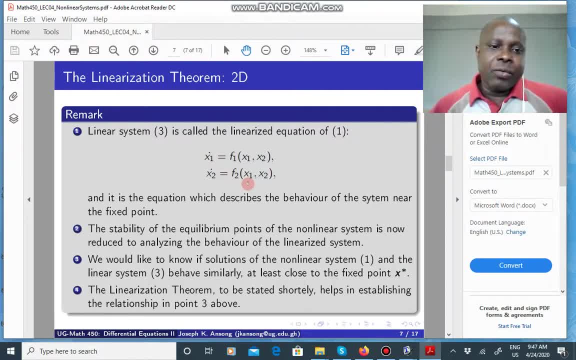 a solution. we don't have the machinery for it. we are now going to analyze the linearized form of it. okay, but by doing that we only know solutions around the fixed point, not the whole plane, unlike the linear systems where we have a solution around the whole plane and we can play around. 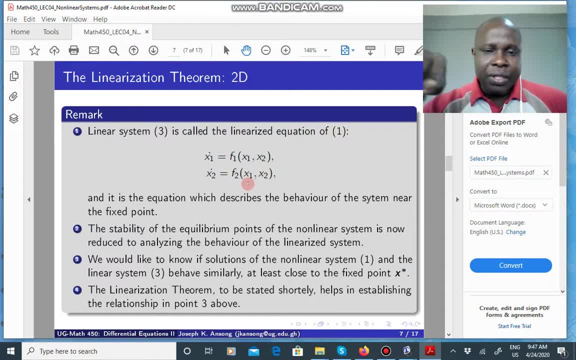 here we can only analyze closer to the fixed point. so that is, that is the limitation, if you like this approach. okay, now, once we familiarize it, want to know whether the behavior that we find around a fixed point is actually the true behavior of the nonlinear system. okay, so that is.